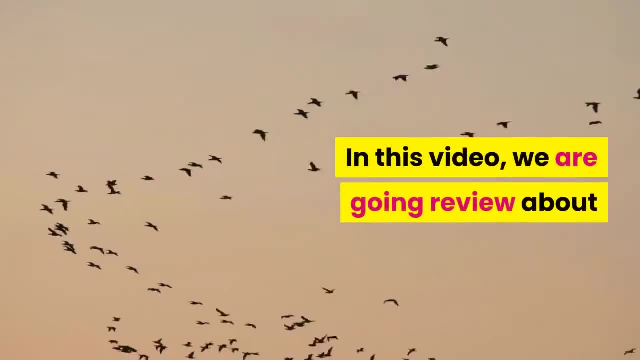 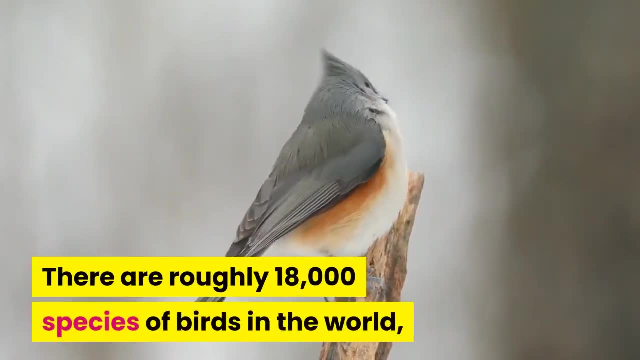 Welcome to TheraPlanet channel. In this video we are going review about The 12 Endangered Birds Most at Risk of Extinction. There are roughly 18,000 species of birds in the world, many of which are at risk of extinction. 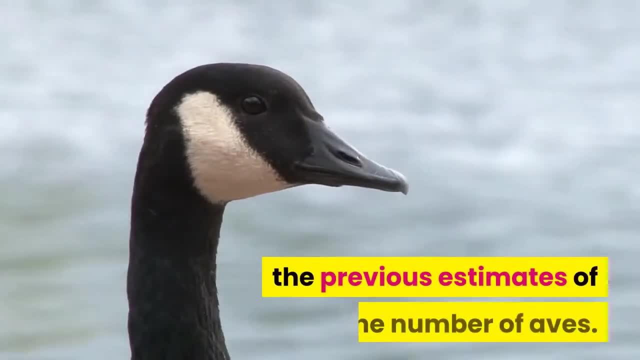 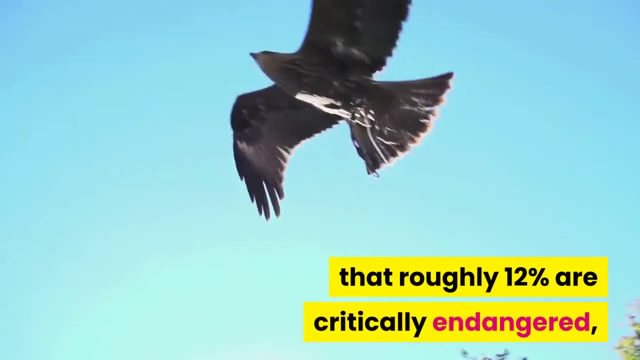 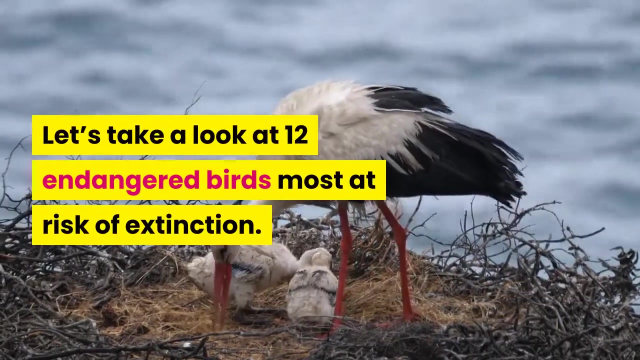 A University of Washington study nearly doubles the previous estimates of the number of aves. Of those birds species estimates predict that roughly 12% are critically endangered- the worst classification before extinct in the wild. Let's take a look at 12 Endangered Birds Most at Risk of Extinction. 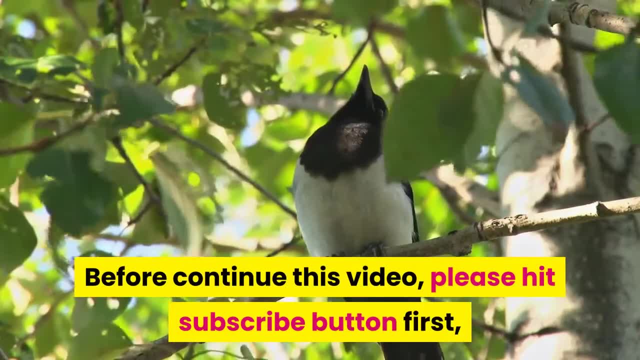 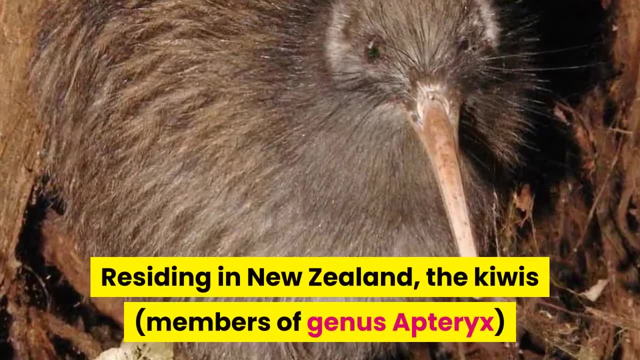 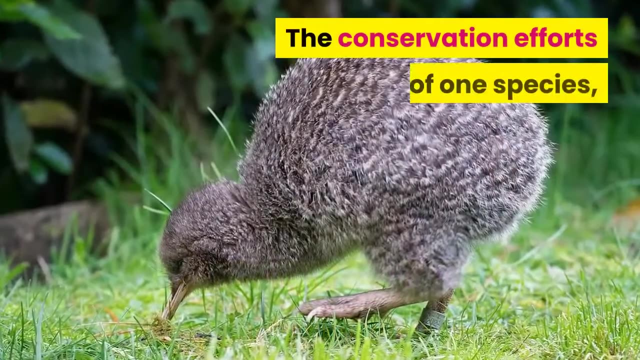 Before continue this video, please hit subscribe button first so you know when we launch new videos. Number 12.. Kiwi Residing in New Zealand. the Kiwis are a group of flightless birds that are endangered and vulnerable. The conservation efforts of one species. 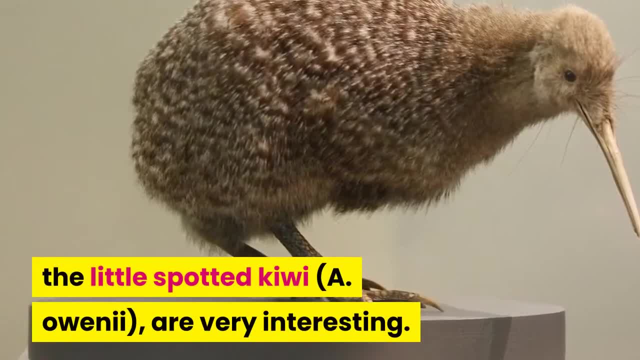 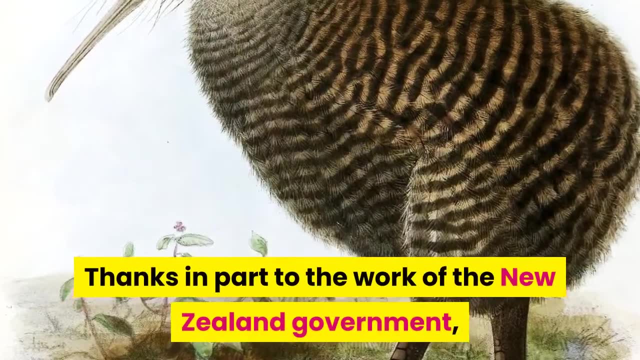 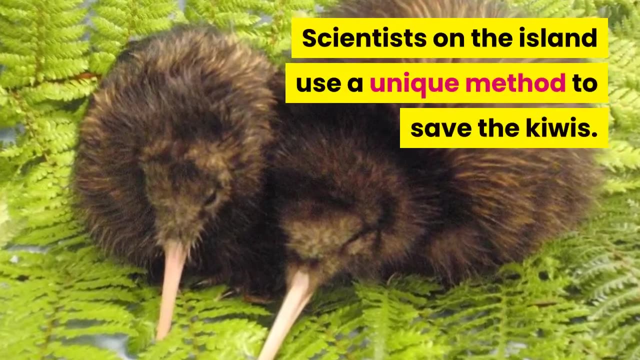 the little spotted kiwi are very interesting. At its low point, the species only had five individuals living. Thanks in part to the work of the New Zealand government, there are now around 1,600 individuals in the wild. Scientists on the island use a unique method to save the kiwis. 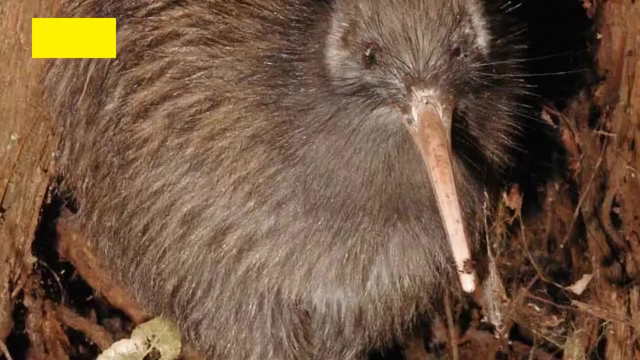 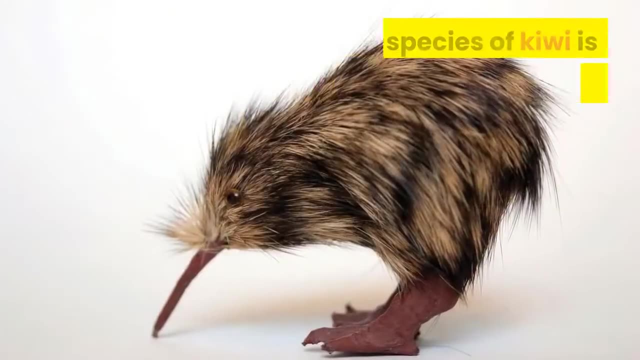 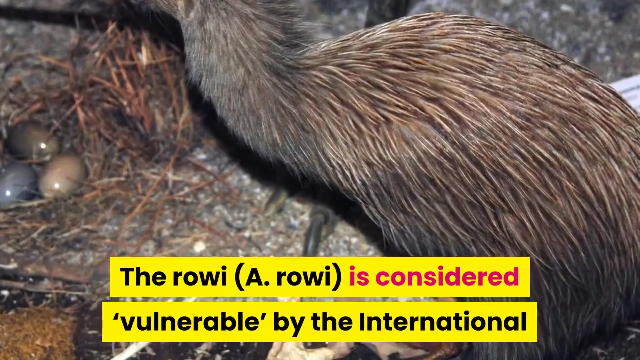 They replace a kiwi's eggs with artificial 3D printed eggs and safely incubate the eggs in a lab. The eggs are returned to the mother when they are ready to hatch. Not every species of kiwi is doing well, though The roe. a roe is considered vulnerable by the International Union for Conservation of Nature. 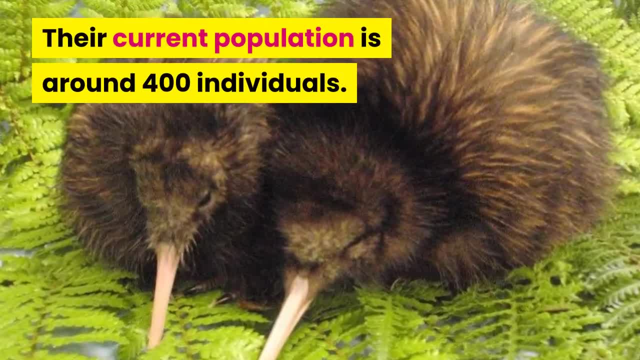 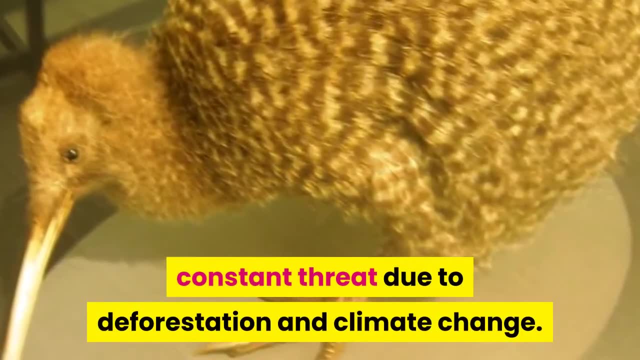 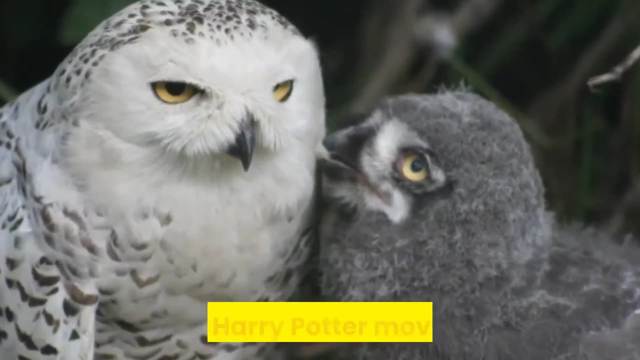 Their current population is around 400 individuals. Unfortunately, the species is under constant threat due to deforestation and climate change. Number 11. Snowy Owl. Most people will recognize the snowy owl b scandiacus from the Harry Potter movie series. 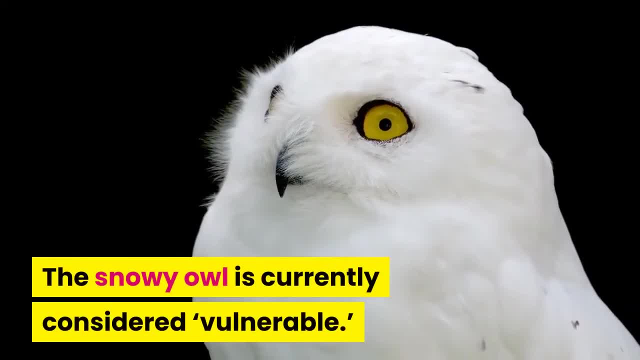 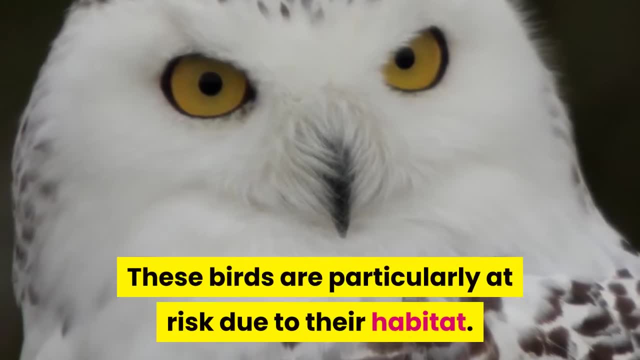 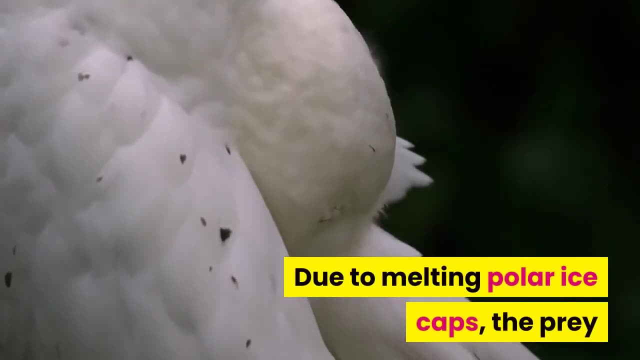 The snowy owl is currently considered vulnerable. what's worse, its population numbers are decreasing rapidly. these birds are particularly at risk due to their habitat. they primarily live north of the 60 degrees latitude line. due to melting polar ice caps, the prey that snowy owls feed on, like mice, are also disappearing, combined with habitat loss, 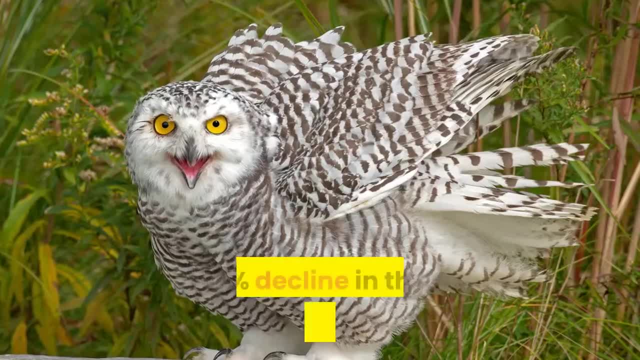 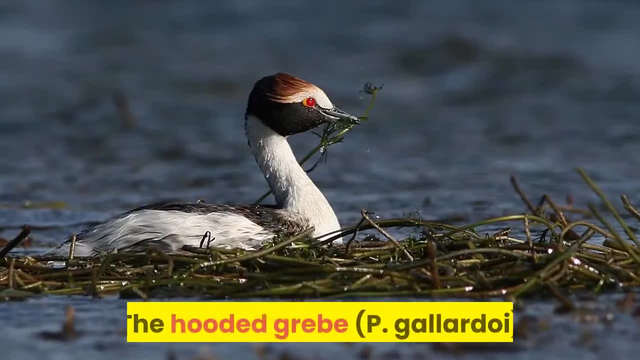 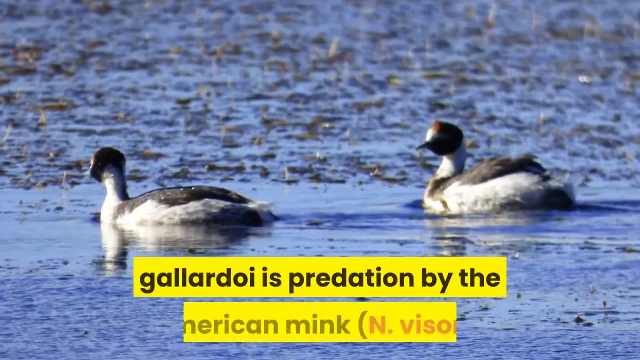 these factors have contributed greatly to the 85% decline in their population since 2003. number 10: hooded grebe. the hooded grebe P galardoi is a bird native to Chilean and Argentinian Patagonia. the main threat to P galardoi is predation by the American mink n v-zone during the first year of. 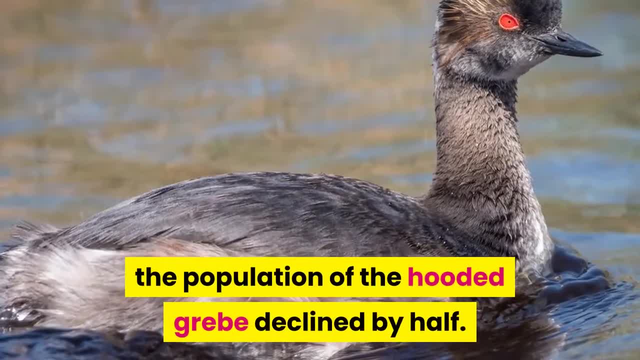 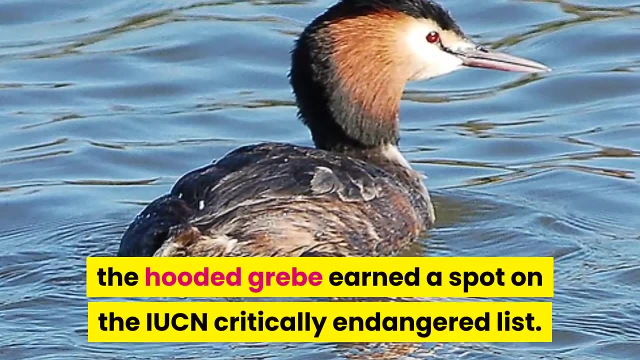 the minks. introduction, the population of the hooded grebe declined by half. due to this decrease, the hooded grebe earned a spot on the IUCN critically endangered list number 9, kakapo. the kakapo, also known as the owl bird, is a bird that lives in the southern part of the United States and is a 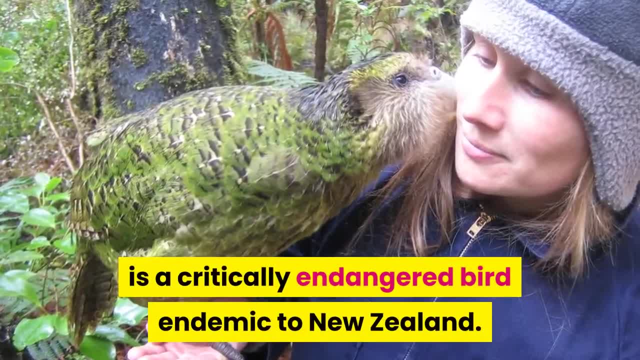 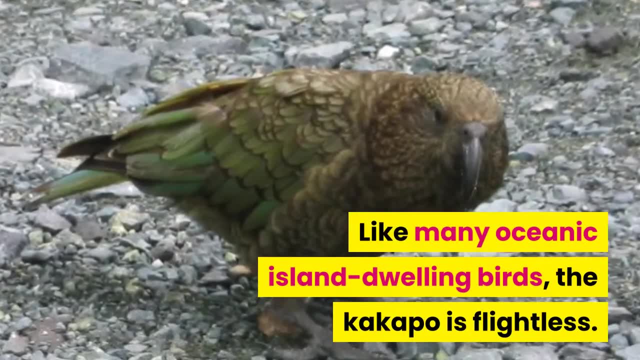 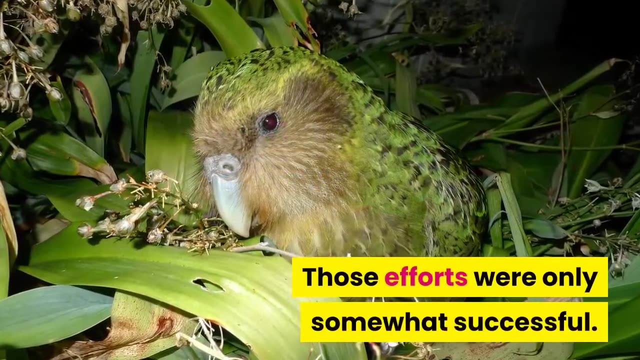 parrott s have reptilis is a critically endangered bird endemic to New Zealand. like many oceanic island-dwelling birds, the kakapo is flightless. conservation efforts began in New Zealand over 125 years ago. those efforts were only somewhat successful. sadly, only 142 individuals are. 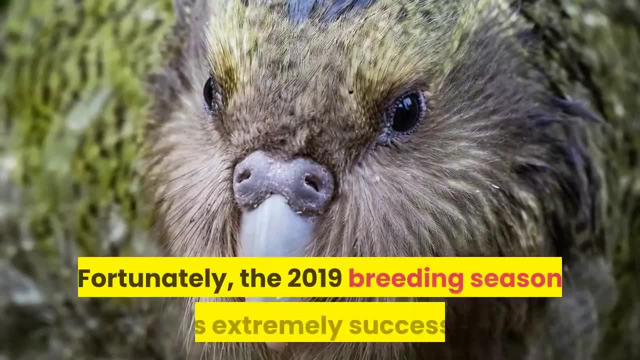 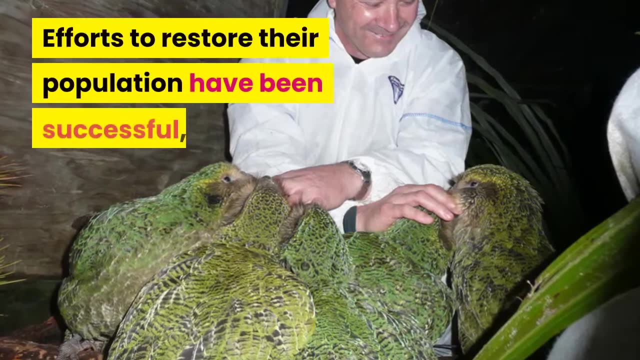 left in the wild as of 2019. fortunately, the 2019 breeding season was extremely successful and 34 chicks are still in the wild. as of 2019, breeding season was extremely successful and 34 chicks are all alive. efforts to restore their population have been successful, but the species still 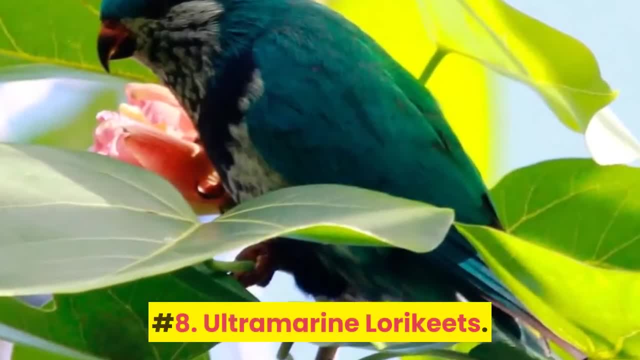 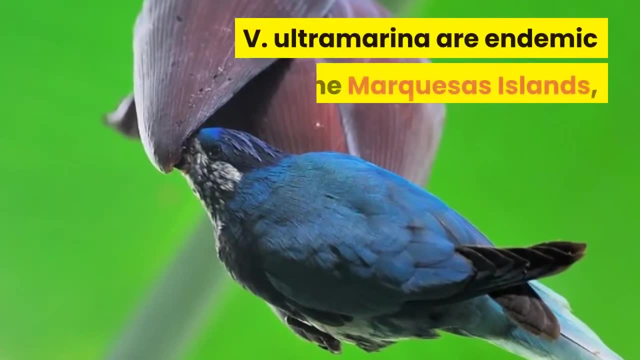 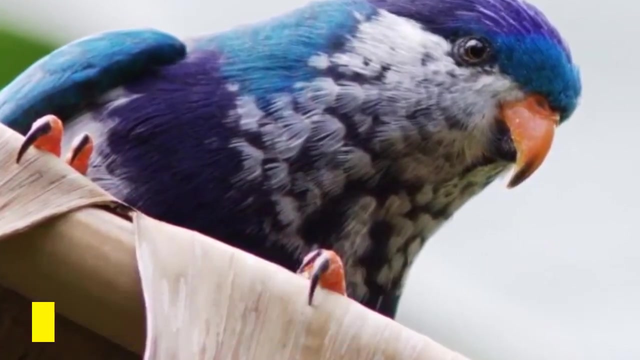 teeters on the brink of extinction. number 8: ultramarine lorikeets. these birds are distinct because of their beautiful coloration. the ultramarina are endemic to the Marcos Islands, an archipelago about 4,800 kilometres, 3,000 miles off the west coast of. 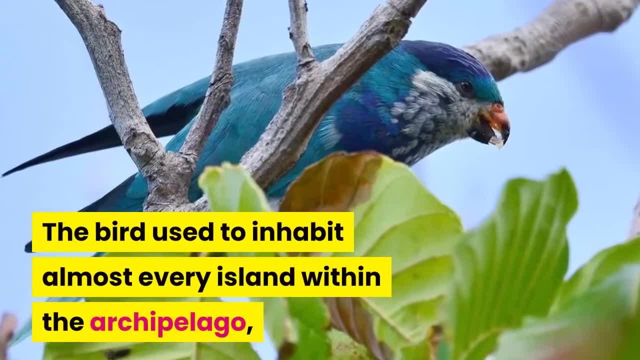 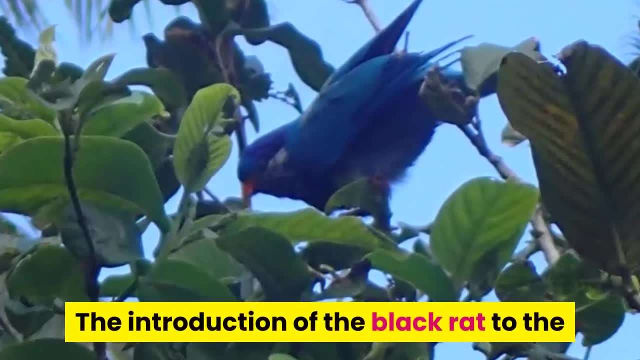 Mexico. The bird used to inhabit almost every island within the archipelago, but now can only be found on the island of Oahuca. The introduction of the black rat to the local ecosystem devastated the population and rendered the lorikeet critically endangered. 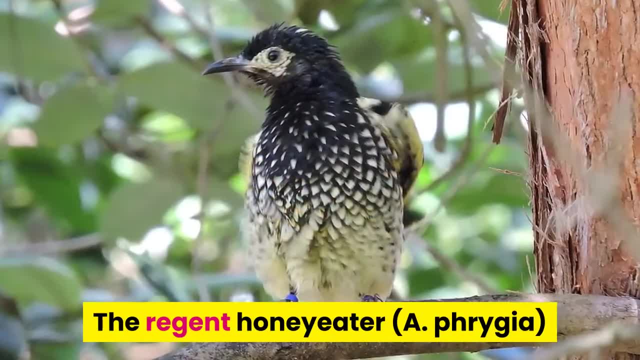 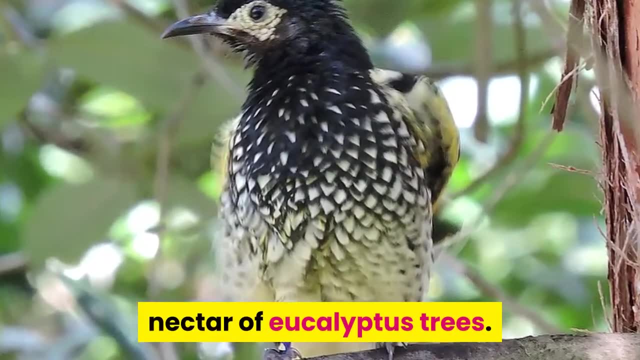 Number 7. Regent Honeyeater. The Regent Honeyeater A frigia gets its name due to one of its preferred food sources: nectar of eucalyptus trees. The bird is native to SE Australia. 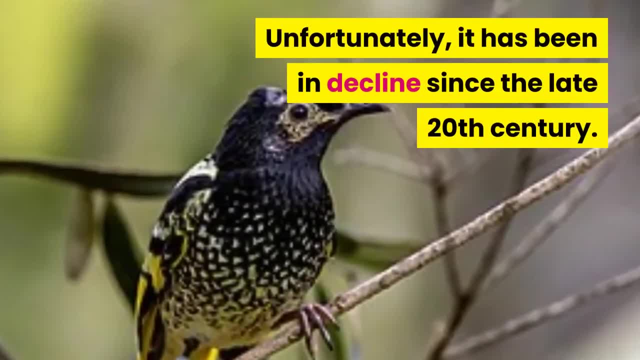 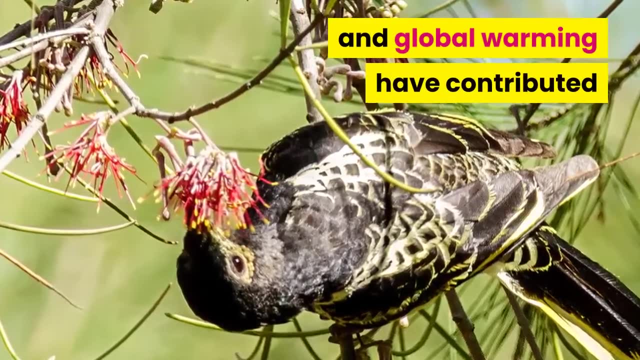 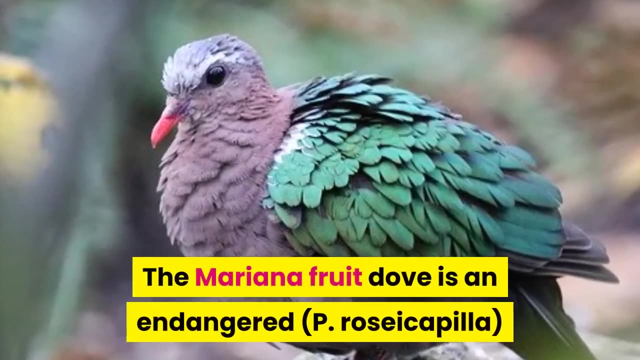 Unfortunately, it has been in decline since the late 20th century. Habitat loss due to the combined effects of human activity and global warming have contributed to their critically endangered status. Number 6. Fruit Dove: The Mariana Fruit Dove is an endangered pea. 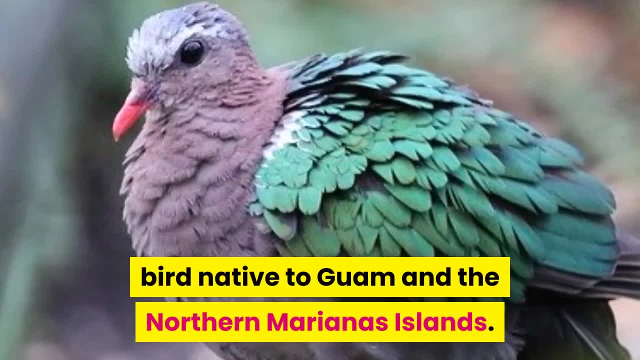 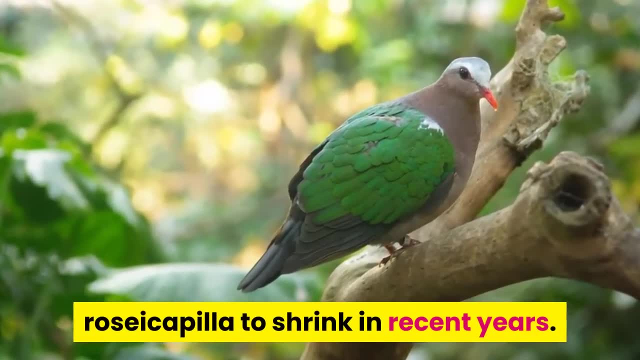 rosicapilla bird native to Guam and the northern Mariana's islands. A host of threats has caused the native population of pea rosicapilla to shrink in recent years. Habitat loss and invasive species are the two largest threats to the rehabilitation of the fruit. 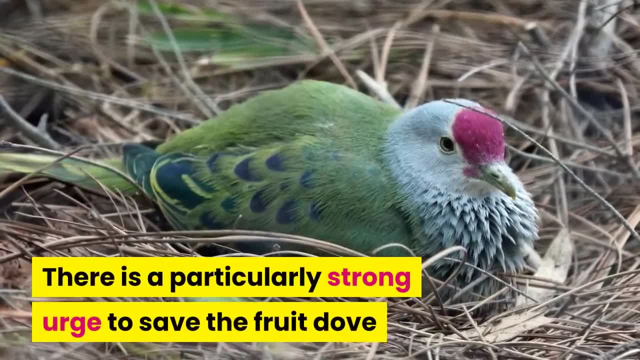 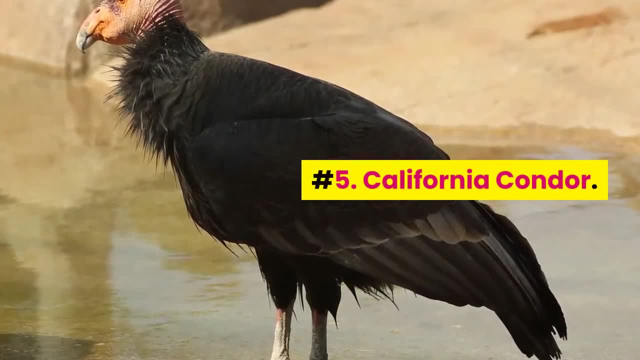 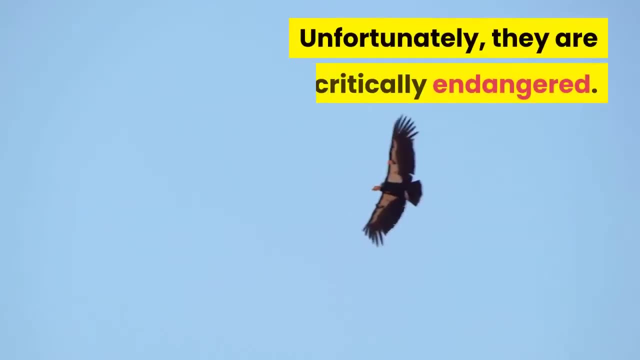 dove. There is a particularly strong urge to save the fruit dove as it is the official bird of the northern Mariana's islands. Number 5. California Condor- Another bird that may be familiar as the California Condor G californianus. Unfortunately, they are critically endangered- The bird actually. went extinct in the wild in 1987.. During the preceding years, the US Department of the Interior, DOI, undertook an ambitious project: to capture every condor left in the wild. At the time, that number was only 26.. Since then, the total 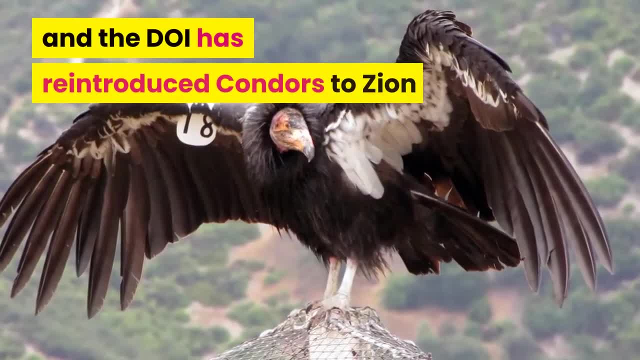 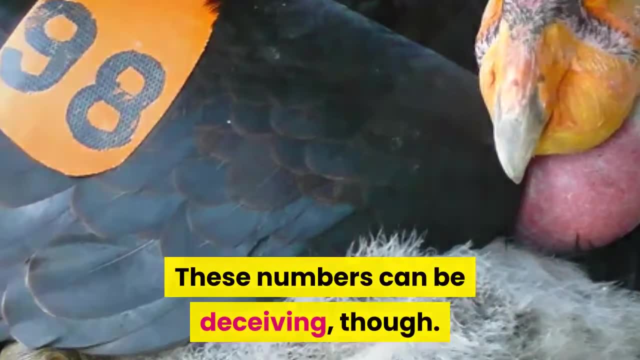 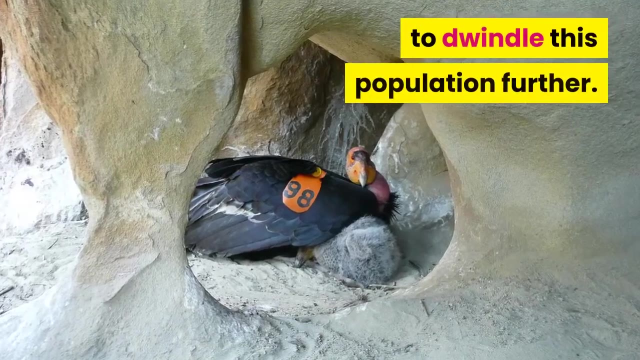 population has risen to over 400, and the DOI has reintroduced condors to Zion and Grand Canyon National Parks. These numbers can be deceiving, though. There are currently only 44 mature individuals in the wild, and even small losses of habitat threaten to dwindle this population further. 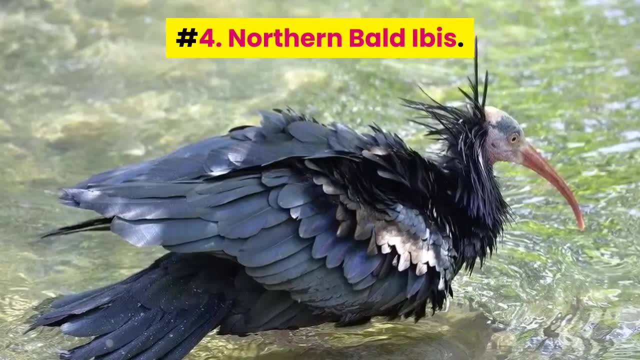 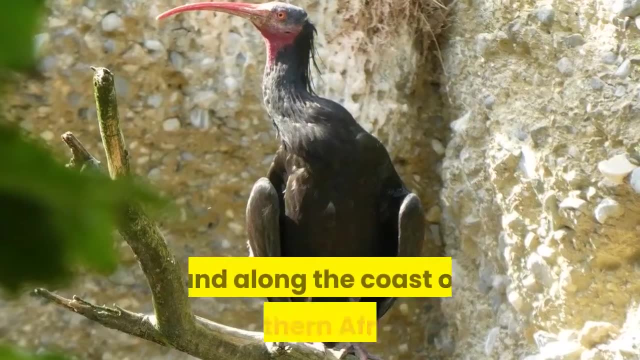 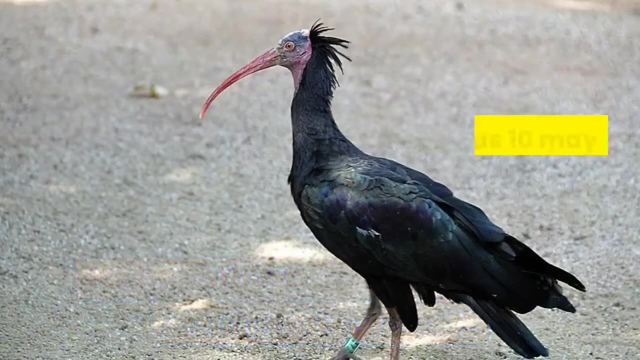 Number 4. Northern Bald Ibis. The reclusive Northern Bald Ibis G aramida lives along the west coast of the Saudi Arabian Peninsula and along the coast of northern Africa. Studies estimate there are less than 500 birds left in the wild Worse as few as the 10th of. 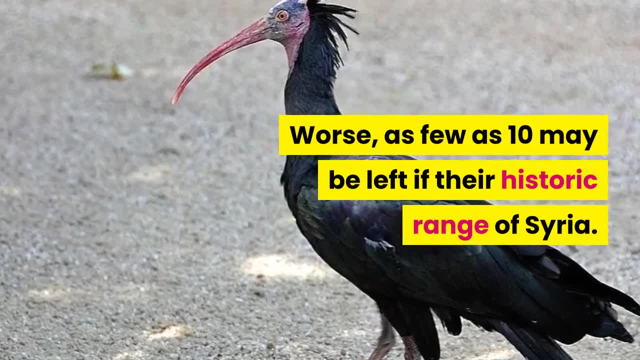 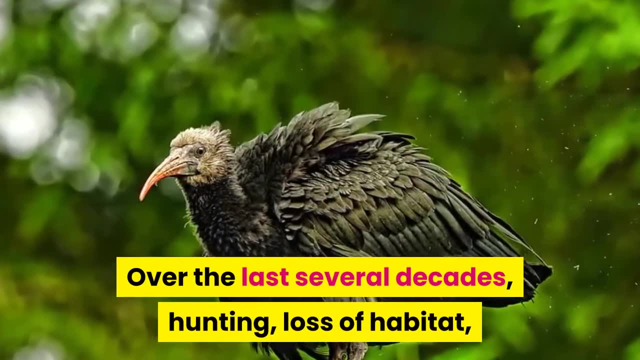 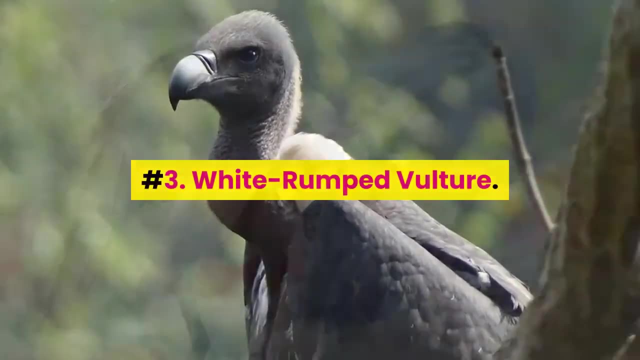 May be left if their historic range of Syria. It is considered to be the rarest bird in the Middle East. Over the last several decades, hunting, loss of habitat and trade have contributed to its current status as endangered Number 3. White-rumped Vulture. At first glance, the listed number of 10,000. 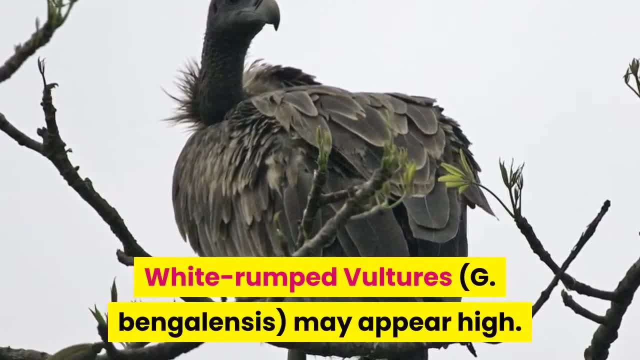 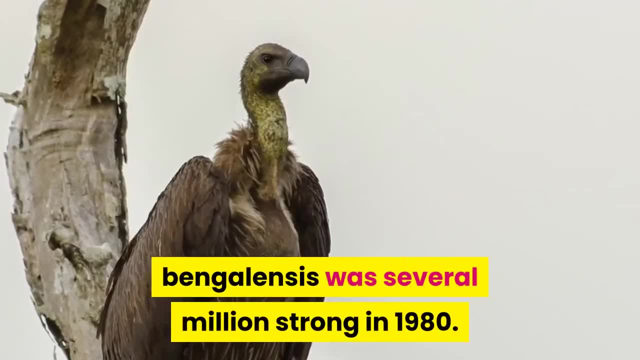 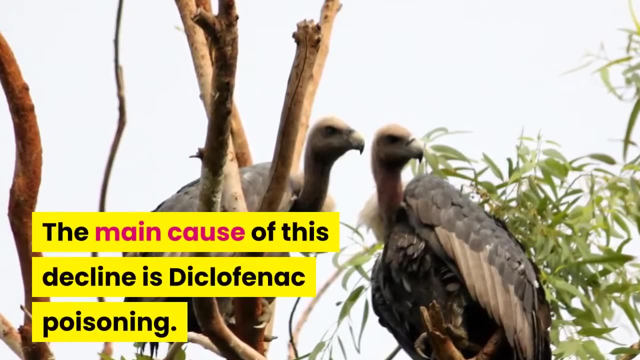 wild white-rumped vultures, G bengalensis, may appear high, But in contrast, the global population of G bengalensis was several million strong in 1980.. At that time, it was one of the most common birds of prey in the world. The main cause of this decline is diclofenac. 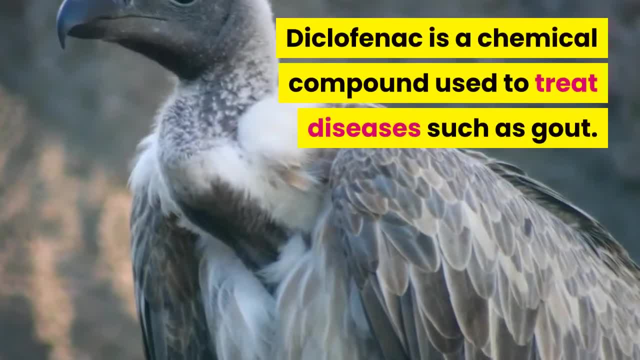 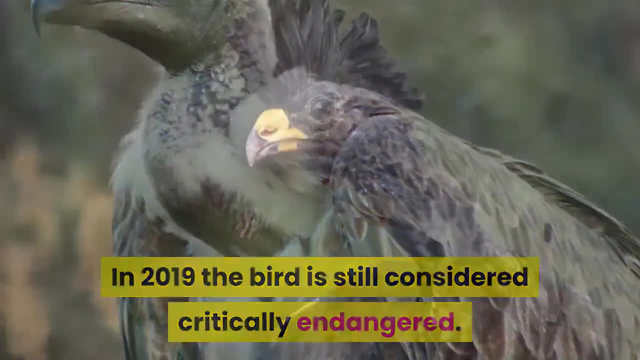 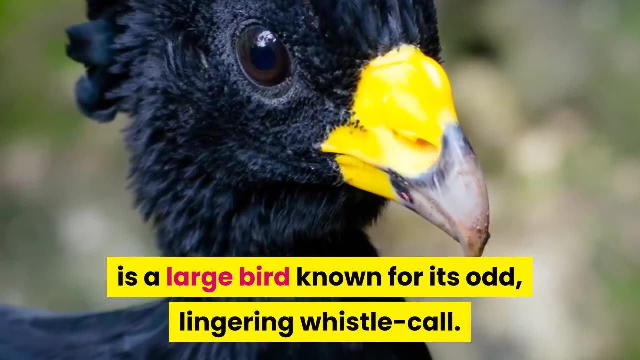 poisoning Diclofenac, chemical compound used to treat diseases such as gout, in 2019, the bird is still considered critically endangered. number two: great carasso. the great carasso see rubra is a large bird known for its odd lingering whistle call. it is a